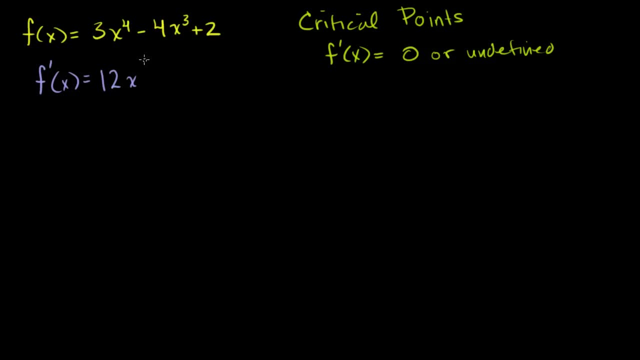 12x to the. we'll just decrement the 4 by 1, 3.. You just multiply times the exponent and then decrease the new exponent by 1, minus 3 times 4 is 12, times x to the. 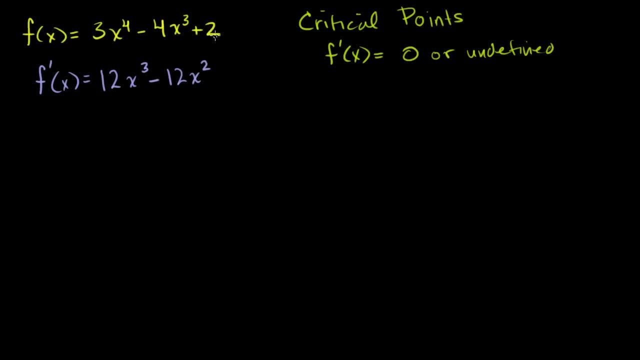 1 less than 3 is 2.. And then the derivative of a constant. the slope of a constant you can almost imagine, is 0. It's not changing. A constant by definition isn't changing. So that's f prime of x. 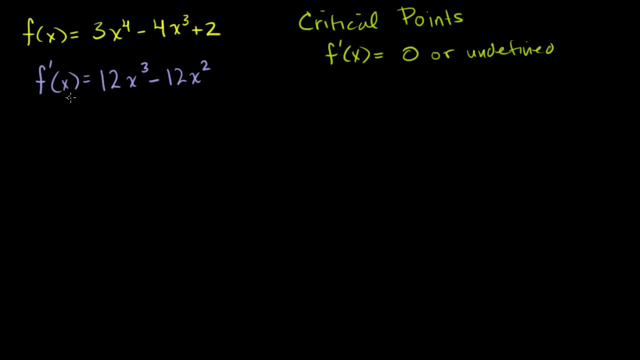 So let's figure out the critical points. The critical points are where this thing is either going to be equal to 0 or it's undefined. Now I could look over the entire domain of real numbers and this thing is defined pretty much anywhere. 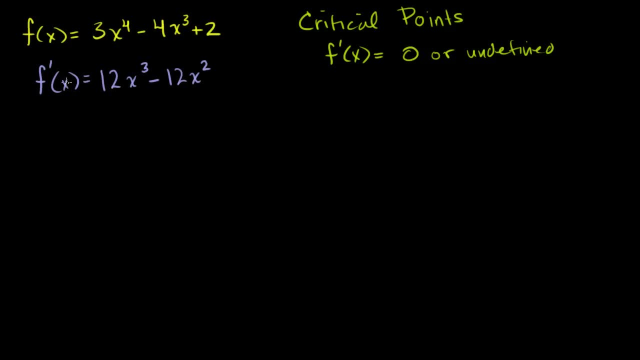 I could put any number here and it's not going to blow up. It's going to give me an answer to what the function is. It's defined everywhere, So let's just figure out where it's equal to 0.. So f prime of x is equal to 0.. 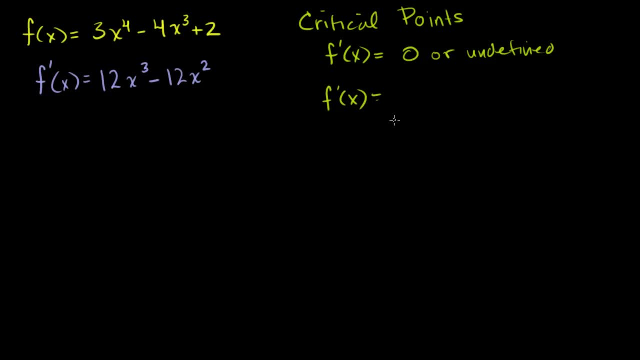 So let's solve which x is. so let's solve. I don't have to rewrite that, I just wrote that Let's solve for whether this is equal to 0.. And I'll do it in the same color. So 12x to the third minus 12x squared is equal to 0.. 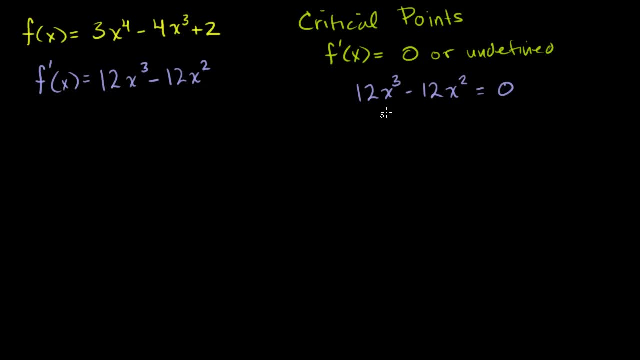 And so let's see what we can do to solve this. Well, we could factor out a 12x. So if we factor out a 12x, then this term becomes just x, And then actually, let's just factor out a 12x squared. 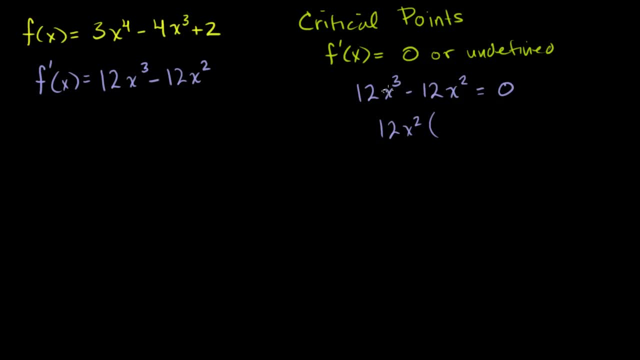 We factor out a 12x squared. If we divide both of these by 12x squared, this term just becomes an x, And then minus 12x squared. divided by 12x squared is just 1, is equal to 0.. 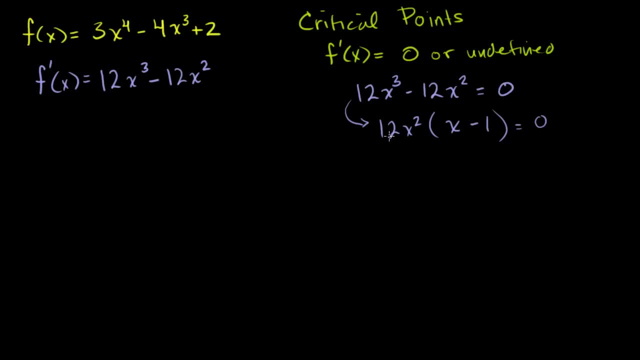 I just rewrote this top thing like this: You could go the other way. If I multiplied, if I distributed this 12x squared times this entire quantity, you would get my derivative right there. So the reason why I did that is because to solve for 0, or. 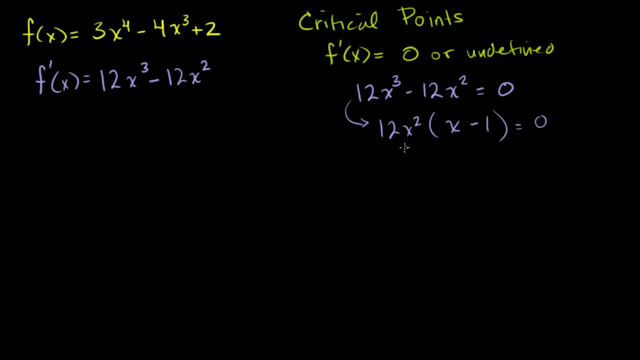 if I want all of the x's that make this equation equal to 0, I now have written it in a form where I'm multiplying one thing by another thing And in order for this to be 0,, one or both of these things. 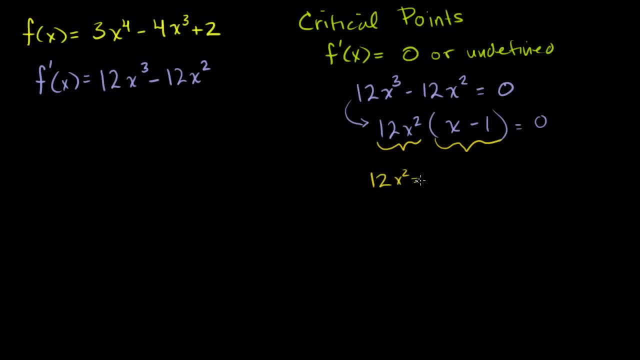 must be equal to 0. So 12x squared are equal to 0, which means that x is equal to 0. So we'll make this quantity equal 0.. And then the other thing that would make this quantity 0 is: 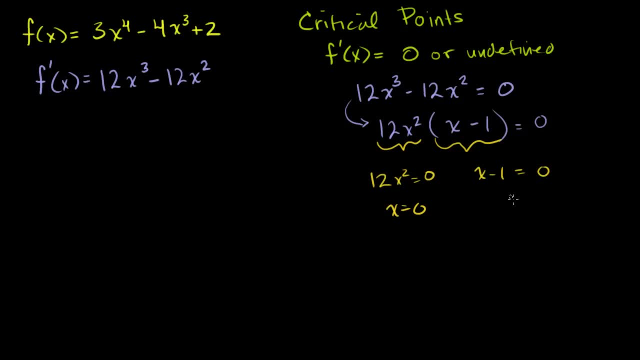 if x minus 1 is equal to 0.. So x minus 1 is equal to 0 when x is equal to 1.. So these are our two critical points. Our two critical points are: x is equal to 0 and x is equal to 1.. 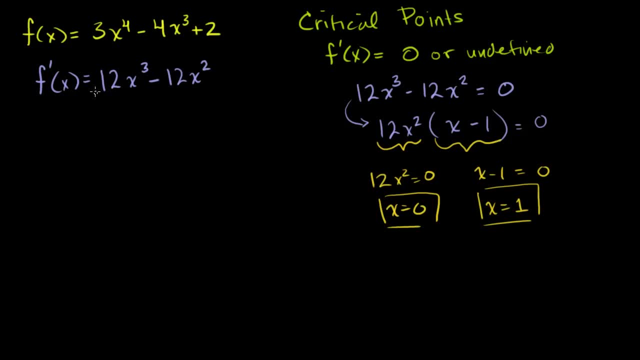 And remember, those are just the points where our first derivative is equal to 0,, where the slope is 0. They might be maximum points, They might be minimum points, They might be inflection points, We don't know. They might be, you know, if this was a constant function? 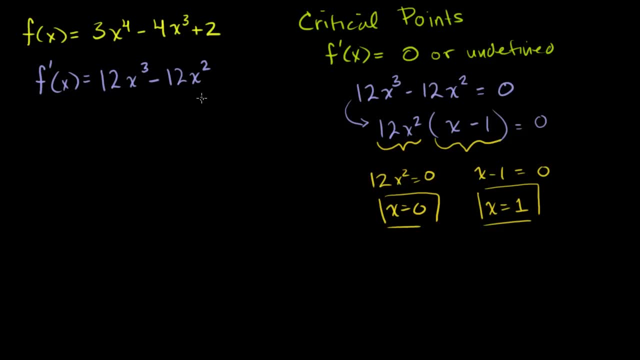 they could just be anything, So we really can't say a lot about them just yet, But they are points of interest. I guess that's all we can say, that they are definitely points of interest, But let's keep going And let's try to understand the concativity. 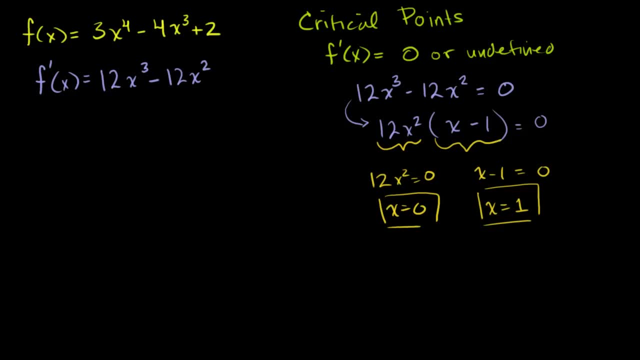 And maybe we can get a better sense of this graph. So let's figure out the second derivative. So the second. I'll do that in. let me do it in this orange color. So the second derivative of minus 1.. My function f. 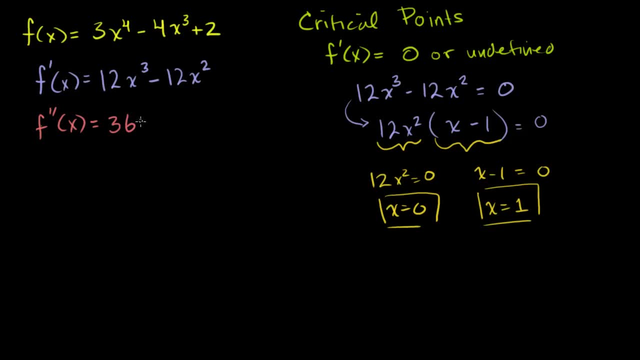 Let's see: 3 times 12 is 36x squared minus 24x. So let's see. well, there's a couple of things we can do Now that we know the second derivative. we can answer the question: is my graph concave upwards? 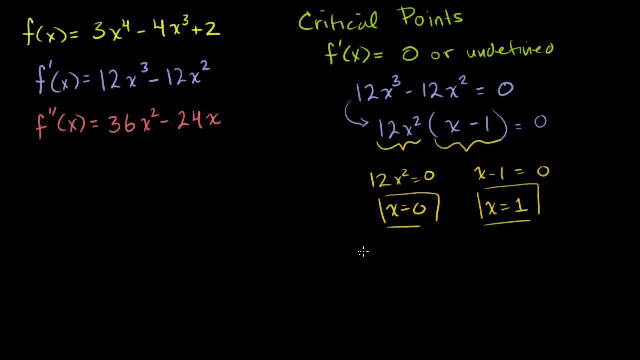 or downwards at either of these points. So let's figure out what at either of these critical points and it'll all fit together. Remember, if it's concave upwards, then we're kind of in a u-shape. If it's concave downwards, then we're. 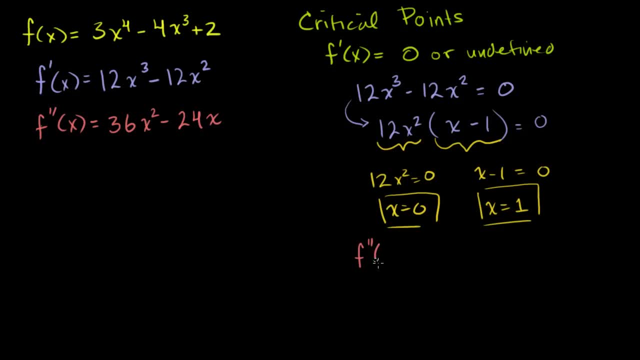 in a kind of upside down u-shape. So f, prime, prime. our second derivative at x is equal to 0, is equal to what It's equal to 36: 0 squared minus 24 times 0. So that's just 0.. 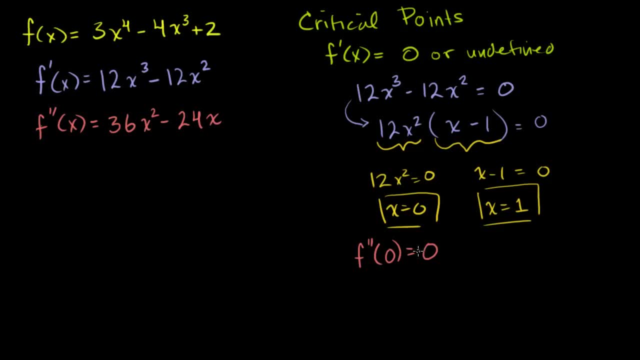 So f, prime, prime. so it's just equal to 0.. So we're in neither concave upwards nor concave downwards here. It might be a transition point, it may not. If it is a transition point, then we're dealing with an inflection point. 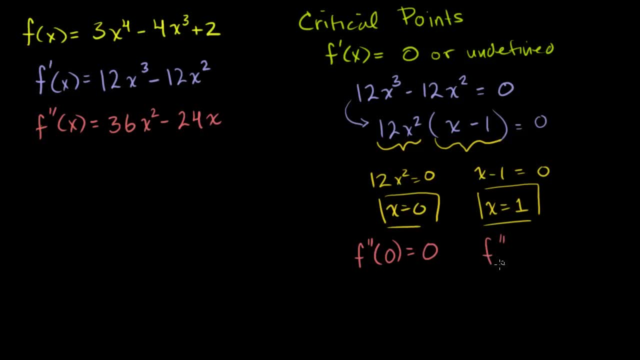 We're not sure yet. Now let's see. Let's see what f, prime, prime or our second derivative, evaluated at 1 is. So that's 36 times 1.. Let me write it down. That's equal to 36 times 1 squared, which is just 36,. 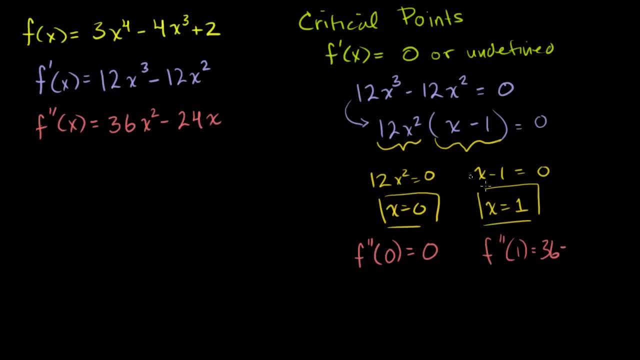 minus 24, minus 24 times 1. So it's 36 minus 24.. So it's equal to 12.. So this is positive. Our second derivative is positive. here It's equal to 12, which means our first derivative. 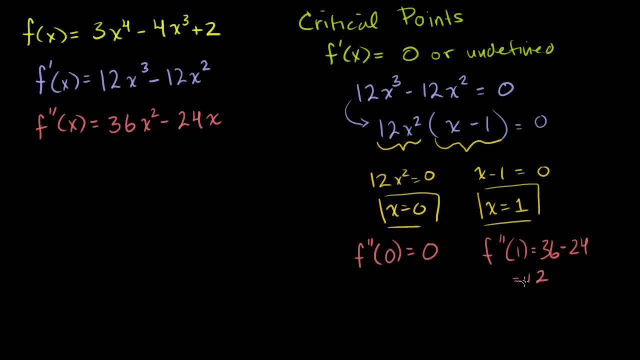 our slope is increasing. The rate of change of our slope is positive here. So at this point, right here, we are concave upwards, which tells me that this is probably a minimum point. The slope is 0 here, but we are concave upwards at that point. 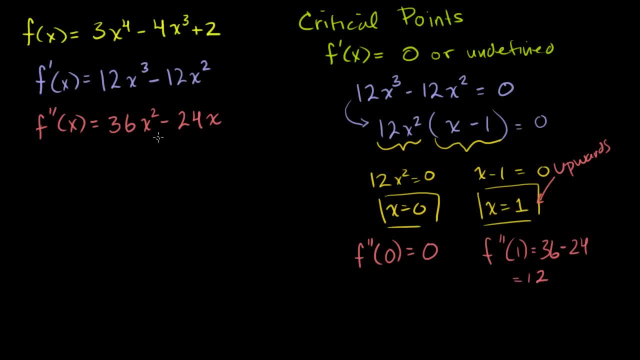 So that's interesting. So let's see if there are any other potential inflection points here. We already know that this is a potential inflection point. Let me circle it in red. It's a potential inflection point. We don't know whether our function actually transitions. 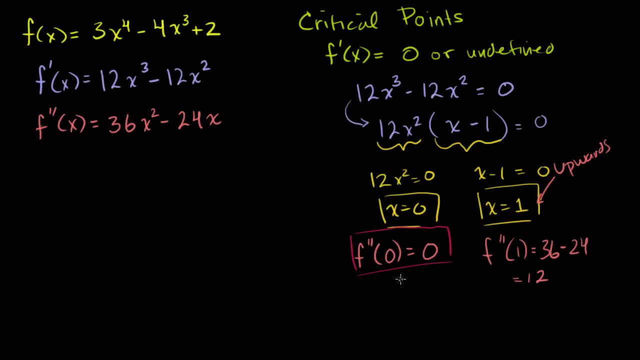 at that point We'll have to experiment a little bit to see if that's really the case. But let's see if there are any other inflection points or potential inflection points. So let's see if this equals 0 anywhere else. 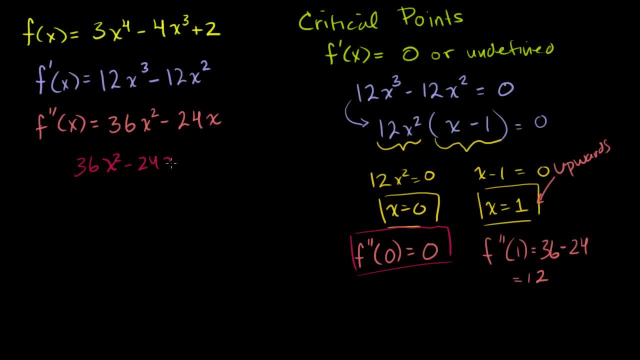 So 36x squared minus 24x is equal to 0.. Let's solve for x. Let us factor out a 12x times 3x. 3x times 12x is 36x squared. So we have a 12x squared minus 2 is equal to 0.. 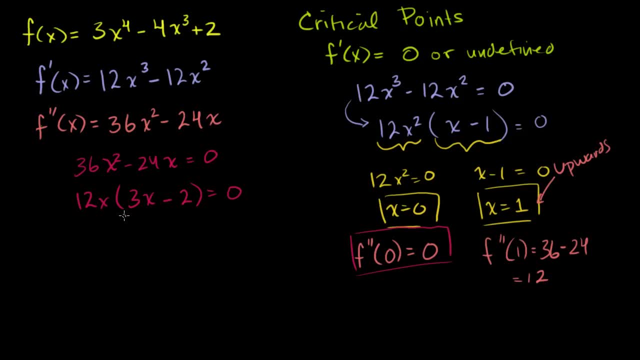 These two are equivalent expressions. If you multiply this out, you'll get this thing up here. So this thing is going to be equal to 0 either, if 12x is equal to 0.. So 12x is equal to 0.. 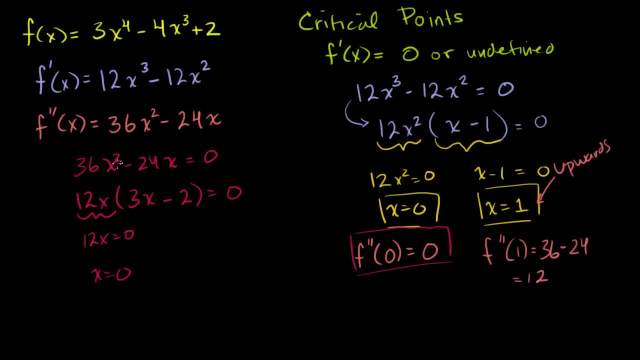 That gives us x is equal to 0. So if x equals 0,, this thing equals 0. So the second derivative is 0 there. And we already knew that because we tested that number out Or this thing. If this expression was 0, then the entire second derivative. 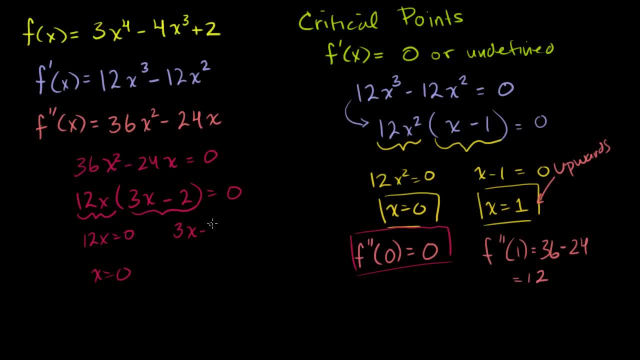 would also be 0. So let's write that. So 3x minus 2 is equal to 0.. 3x is equal to 2.. Just adding 2 to both sides, 3x is equal to 2 thirds. 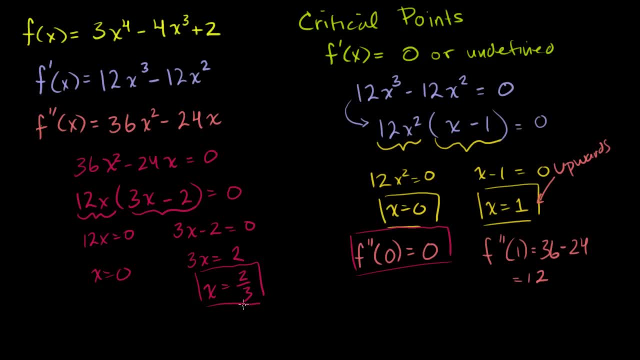 So this is another interesting point that we haven't really hit upon before. that might be an inflection point, And the reason why I say it might be is because the second derivative is definitely 0. here You put 2 thirds, here you're going to get 0.. 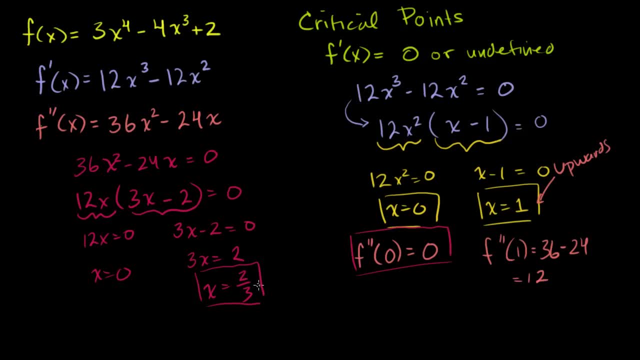 And what we have to do is see whether the second derivative is positive or negative on either sides of 2 thirds, And we already have a sense of that. We could try out a couple of numbers. We know that if we say that x is greater than 2 thirds, 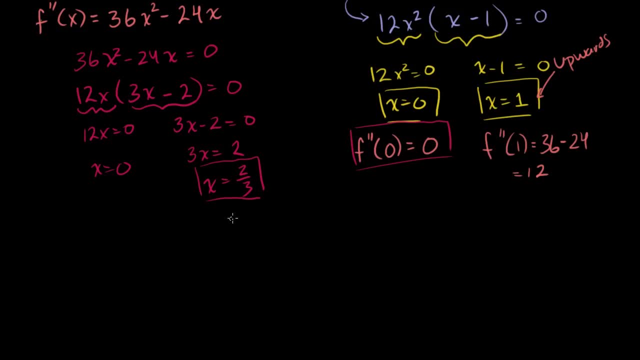 Let me scroll down a little bit, just so we have some space. So let's see what happens When x is greater than 2 thirds: what is f prime of x? So let's see, Sorry, what is f prime prime. 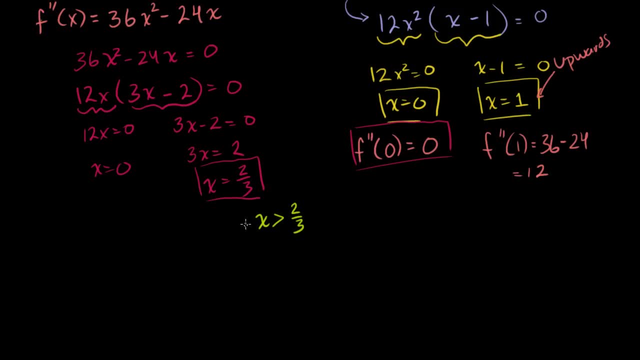 What is the second derivative? So let's try out a value that's pretty good, Pretty close, just to get a sense of things. Just to get a sense of things. So let me rewrite it: f prime prime of x is equal to. let me write it like this: 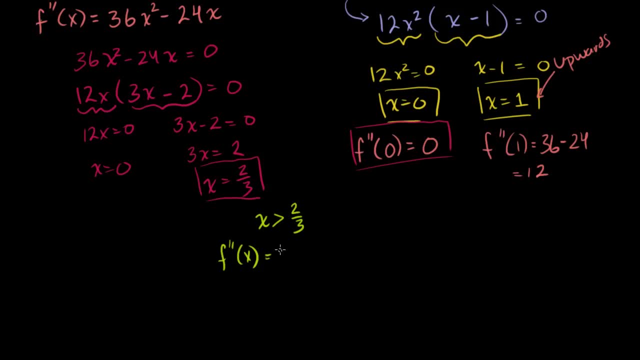 I mean I could write it like this, but this might be easier to deal with- It's equal to 12x times 3x minus 2.. So if x is greater than 2 thirds, this term right here is going to be positive. 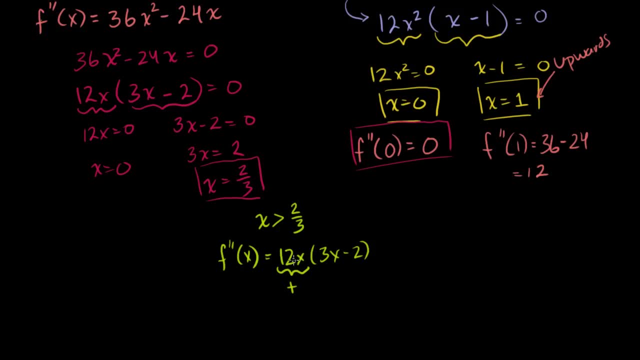 That's definitely. you know, any positive number times 12 is going to be positive. But what about this term right here? 3 times 2, thirds minus 2 is exactly 0, right, That's 2 minus 2.. 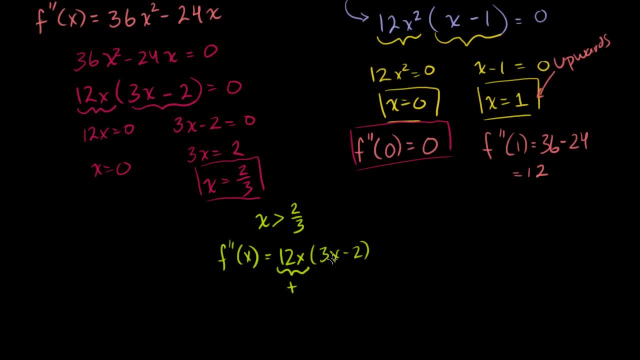 But anything larger than that, 3 times, you know, if I had 2.1 thirds here, this is going to be a positive quantity. Any value of x greater than 2 thirds will make this thing right here, positive right. 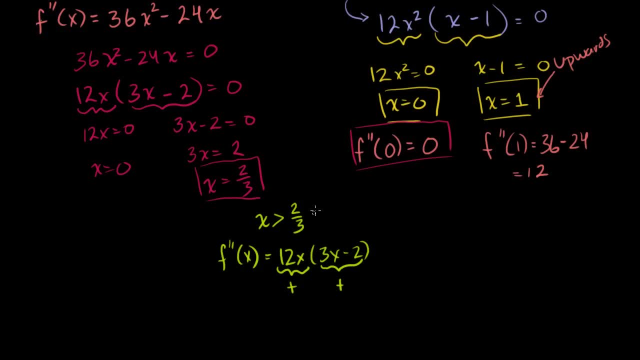 This thing is also going to be positive. So that means that when x is greater than 2 thirds, that tells us that the second derivative is positive. It is greater than 0. So in our domain, as long as x is larger than 2 thirds, we are. 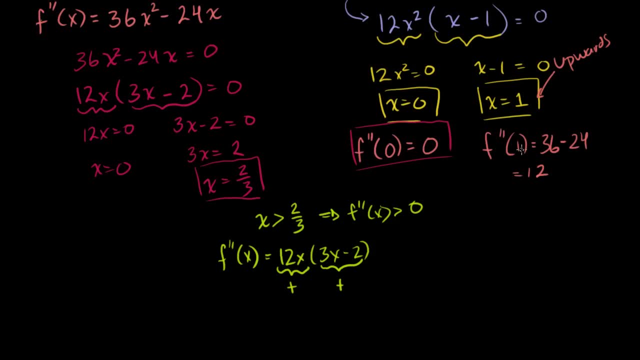 concave upwards And we saw that here, At x is equal to 1, we were concave upwards, But what about x being less than 2 thirds? So when x is less than 2 thirds, let me write it, let me. 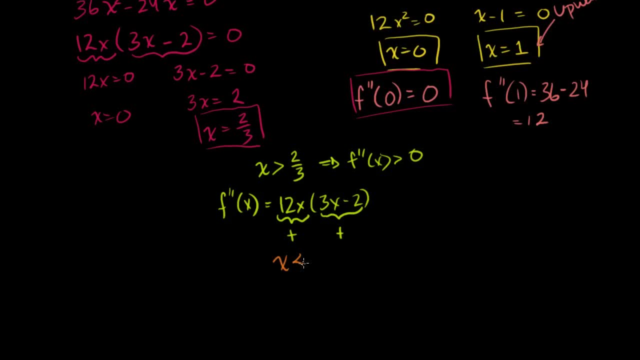 scroll down a little bit. When x is less than 2 thirds, what's going on? I'll rewrite it. f prime, prime of x, second derivative, 12x Times 3x minus 2.. Well, if it goes really far less, we're going to get a. 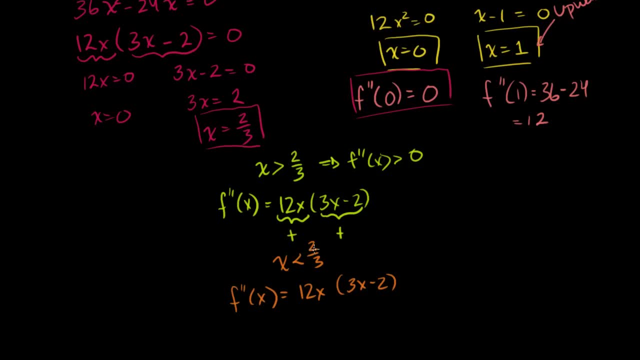 negative number here. And this might be negative, But let's see, if we just go really right below 2 thirds, We're still in the positive domain. So if this was like 1.9 thirds, which is a mixture of a decimal and a fraction, or even 1 third, this thing is. 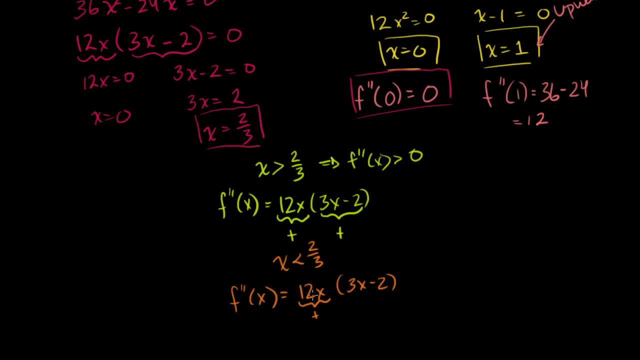 still going to be positive. Right below 2 thirds. this thing is still going to be positive. We're going to be multiplying 12 by a positive number. But what's going on right here? What's going on right here? At 2 thirds, we're exactly 0.. 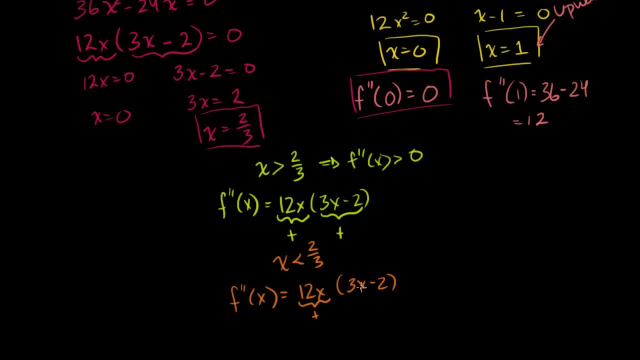 But as you go, as anything less than 2 thirds 3 times 1 third is only 1.. 1 minus 2, you're going to get negative numbers. So when x is less than 2 thirds, this thing right here. 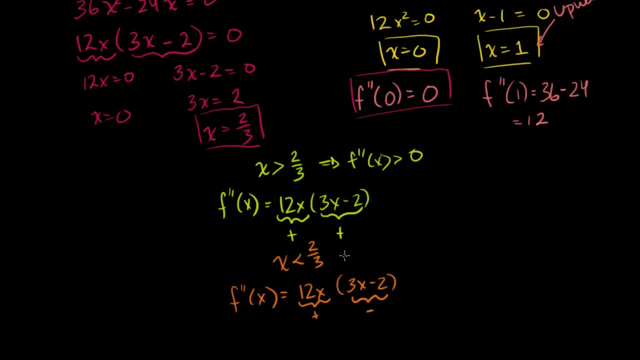 is going to be negative. So the second derivative, if x is less than 2 thirds, the second derivative, right to the left or right, when you go less than 2 thirds, the second derivative of x is less than 0.. Now, the fact that we have this transition from when we're less, 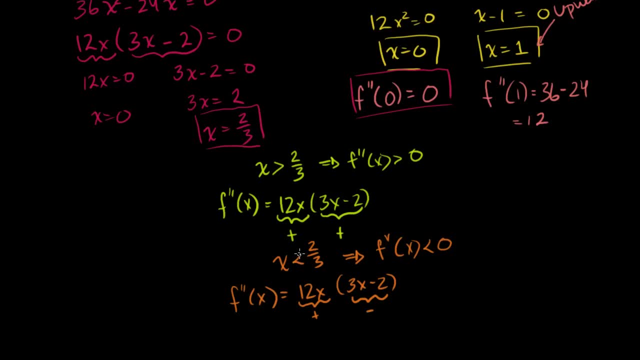 than 2 thirds, we have a negative second derivative, And when we're greater than 2 thirds, we have a positive second derivative. That tells us that this, indeed, is an inflection point. That x is equal to 2 thirds is definitely an inflection point. 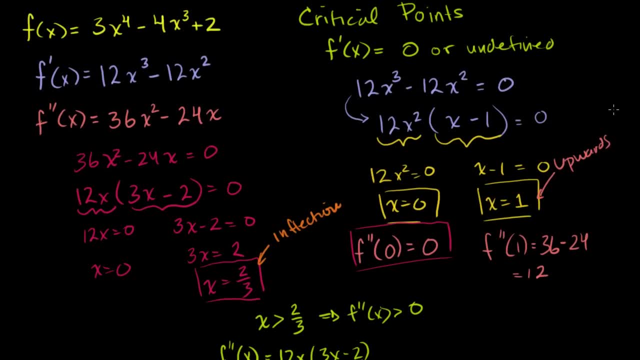 for our original function up here. Now we have one more candidate inflection point And then we're ready to graph. Then, once you know all the inflection points and the maximum minimum, you are ready to graph the function. So let's see: if x is equal to 0 is an inflection point. 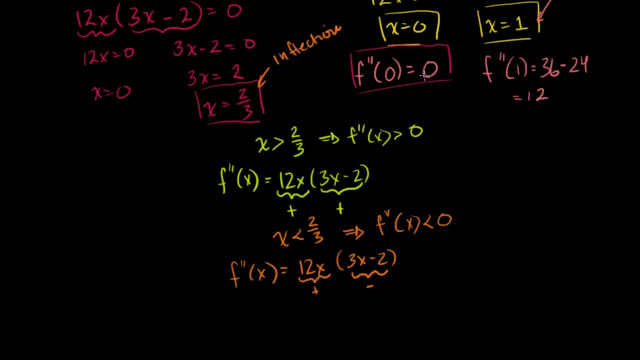 We know that the second derivative is 0 at 0. But what happens above and below the second derivative? So let me do our little test here. So when x is, let me draw a line so we don't get confused with all of the stuff that I wrote here. 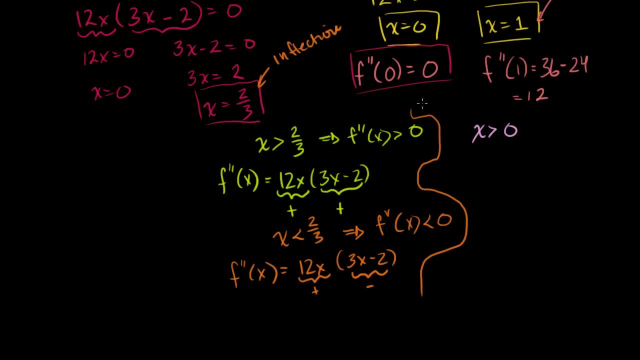 So when x is greater than 0, what's happening to the second derivative? Remember, the second derivative was equal to 12x times 3x squared Minus 2.. I like writing it this way because you've kind of decomposed it into two linear expressions. 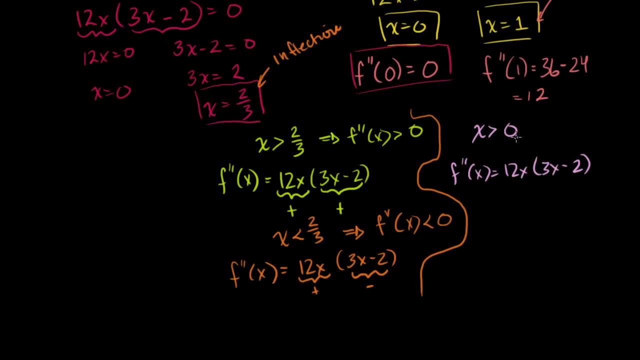 And you could see whether each of them are positive or negative. So if x is greater than 0, this thing right here is definitely going to be positive. And then this thing right here, right, when you go right above, x is greater than 0.. 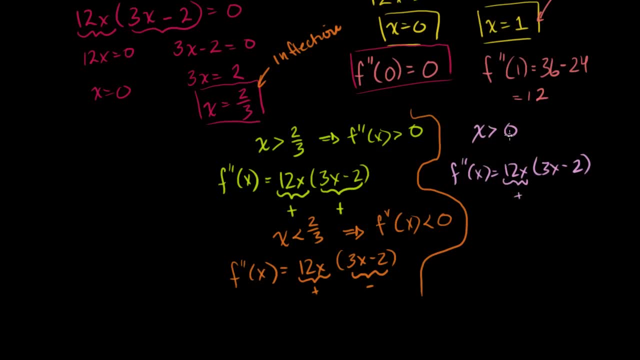 So we have to make sure to be very close to this number. So if this number is like point, let's say it's 0.1.. So you're right above 0. So this isn't going to be true for all of x. 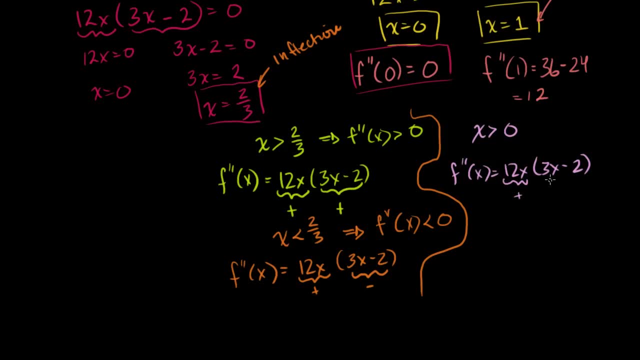 It's greater than 0. We just want to test exactly what happens right when we go right above 0. So if this was 0.1, you would have 0.3.. 0.3 minus 2, that would be a negative number. 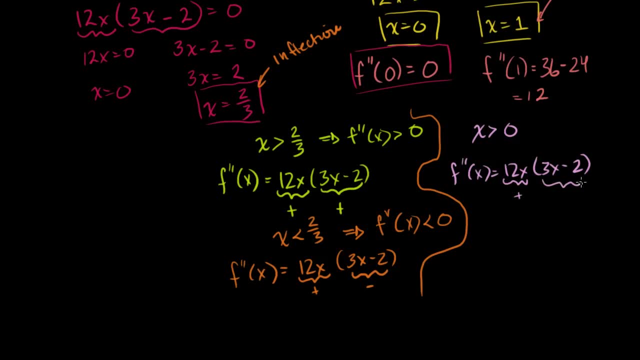 So, right as x goes right above 0, this thing right here is negative. So as x is greater than 0, you will have your second derivative is going to be less than 0. You're concave downwards, Which makes sense, because at some point we're going to be. 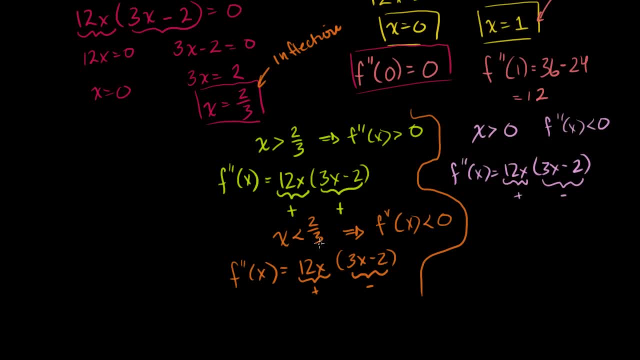 hitting a transition. Remember we were concave downwards before we got to 2 thirds, right. So this is consistent: From 0 to 2 thirds we are concave downwards And then at 2 thirds we become concave upwards. 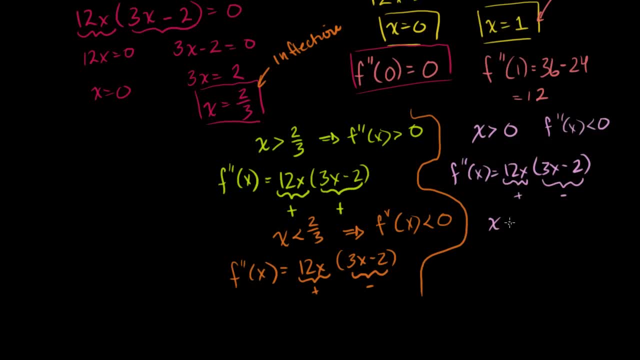 Now let's see what happens when x is just barely less than 0. So, once again, f prime. the second derivative of x is equal to 12x times 3x minus 2.. Well right, if x was minus 0.1 or minus 0.001,. 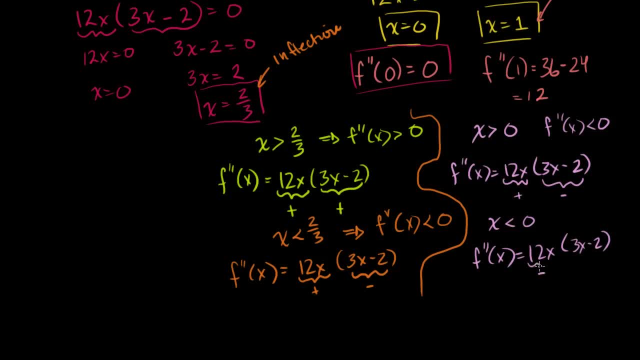 no matter what, this thing is going to be negative. This expression right here is going to be negative. The 12x right. You have some negative value here. Times 12 is going to be negative, And then what's this going to be? 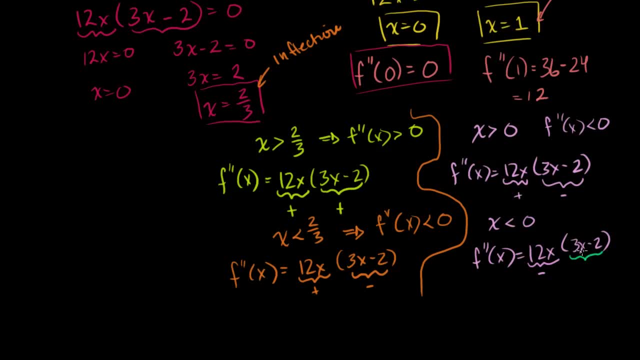 Well, 3 times minus 0.1 is going to be minus 0.3.. Minus 2 is minus 2.3.. You're definitely going to have a negative. This value right here is going to be negative And then when you subtract from a negative, it's definitely. 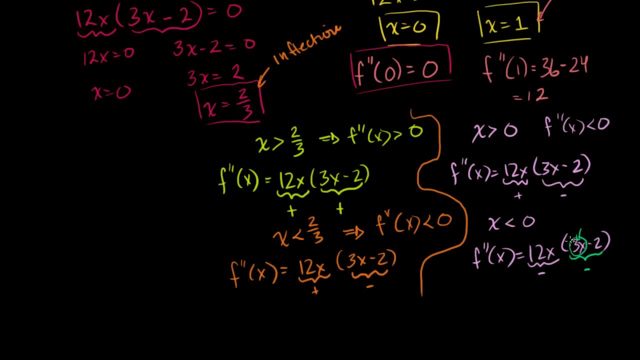 going to be negative. So that is also going to be negative. But if you multiply a negative times a negative, you're going to get a positive. So actually, right below x is less than 0,. the second derivative is positive. Now, this all might have been a little bit confusing, but we 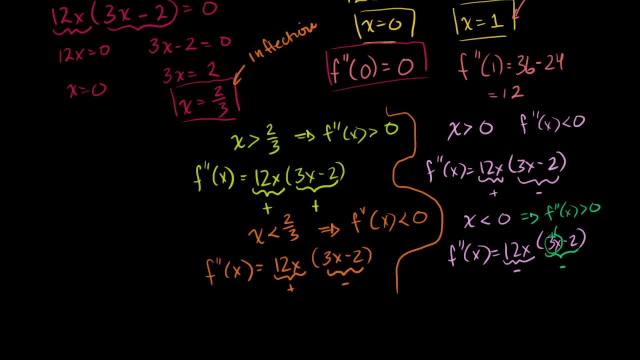 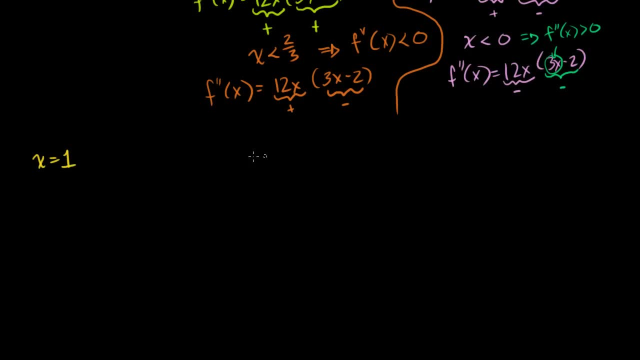 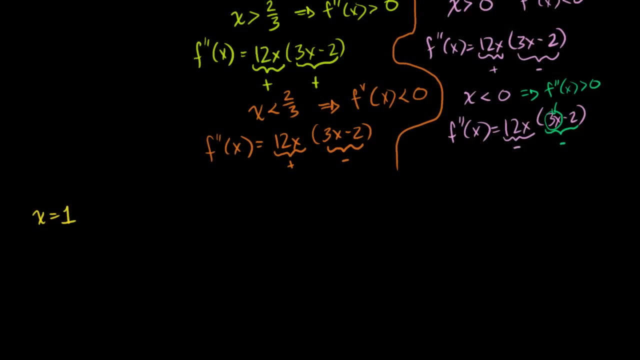 should now have the payoff. We have all of the interesting things going on. We know that at x is equal to 1, let me write it over here. We figured out: at x is equal to 1, the slope is 0. 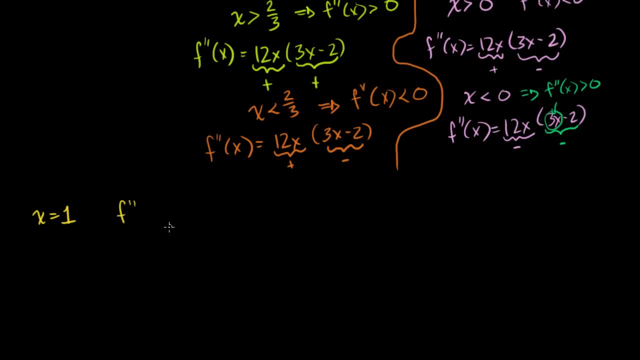 So f prime, prime is sorry, let me write it this way. I should have said: we know that the slope is 0.. Slope is equal to 0. And we figured that out because the first derivative was 0. This was a critical point. 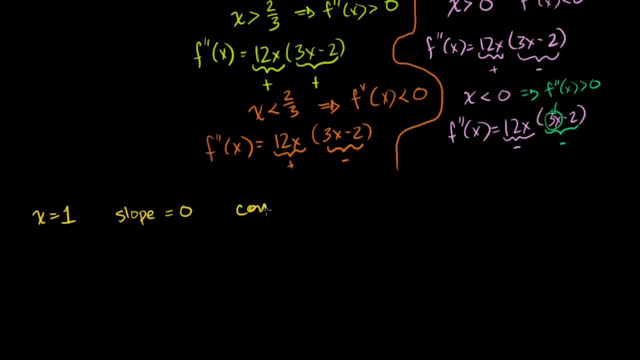 And we know that we're dealing with. the function is concave upwards at this point And that tells us that this is going to be a minimum point. So what is f of? and we should actually get the coordinates so we can actually graph. 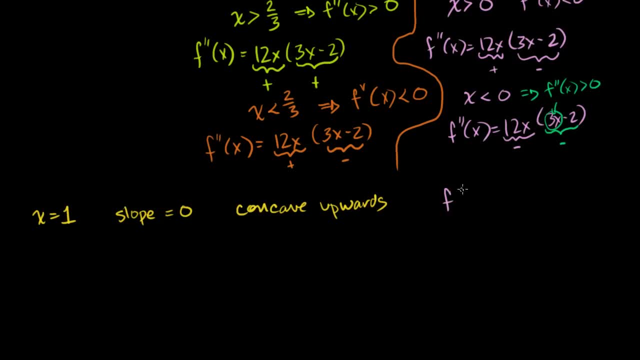 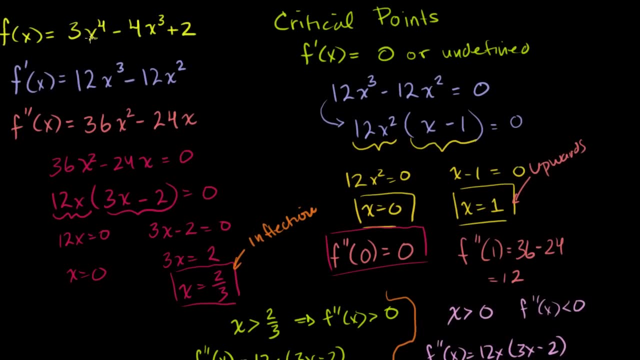 That was the whole point of this video. So, and f of 1 is equal to what f of 1, let's go back to our original function is 3 times 1, right, 1 to the fourth is just 1.. 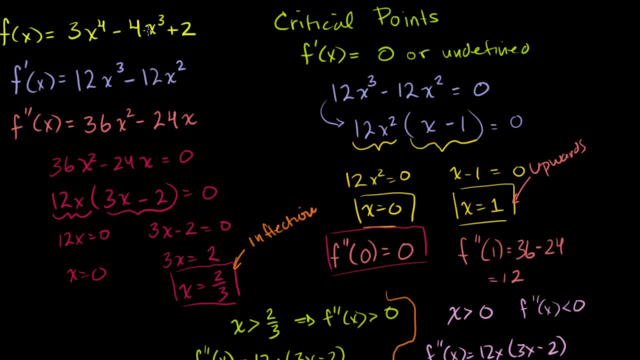 3 times 1 minus 4 plus 2, right, So 4 times. so it's well 3 times 1 minus 4 times 1, which is minus 1, plus 2.. Well, that's just a positive 1.. 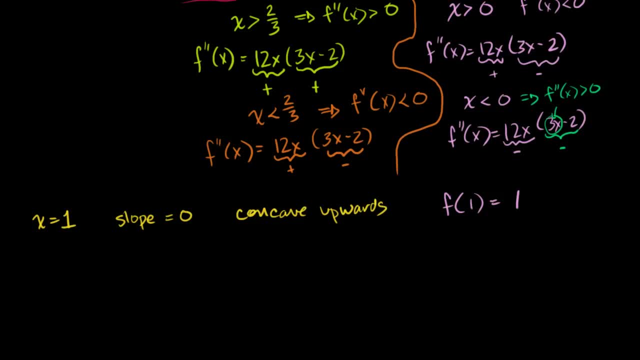 So f of 1 is 1.. And then we know At x is equal to 0, we also figured out that the slope is equal to 0. But we figured out that this was an inflection point. right, The concavity switches before and after. 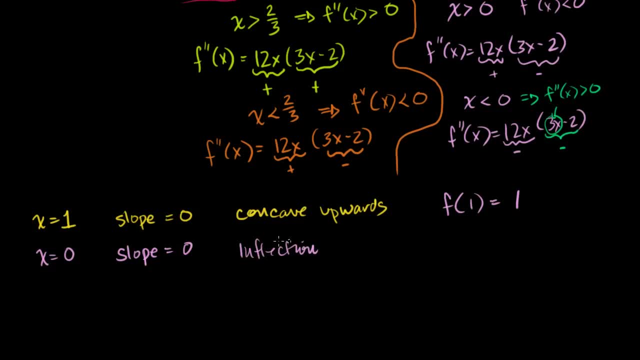 So this is an inflection point And we are concave below 0.. So when x is less than 0, we are upwards, Our second derivative is positive, And when x is greater than 0, we are downwards. We are concave downwards. 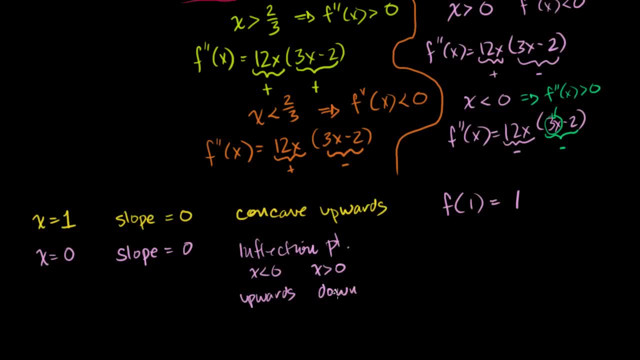 Right above, Not for all of the domain- x and 0, just right above 0.. Downwards. And then what is f of 0?? Just so we know. so we want to graph that point: f of 0.. Let's see f of 0, this is easy. 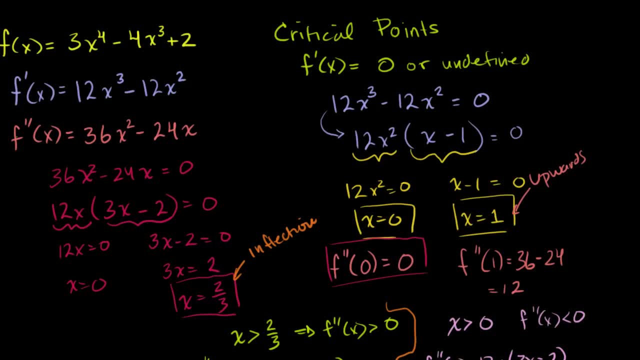 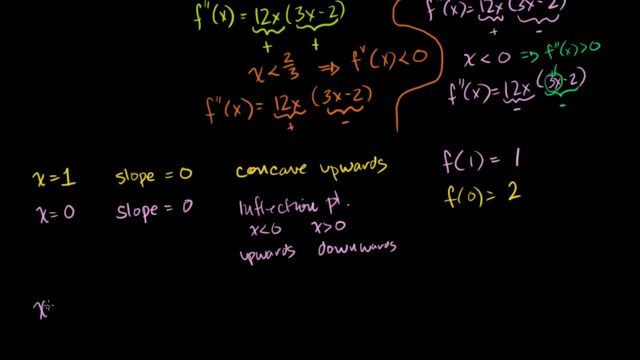 3 times 0 minus 4 times 0 plus 2.. Well, that's just 2.. f of 0 is 2.. And then finally we got the point: x is equal to 2 thirds. x is equal to. let me do that in another color. 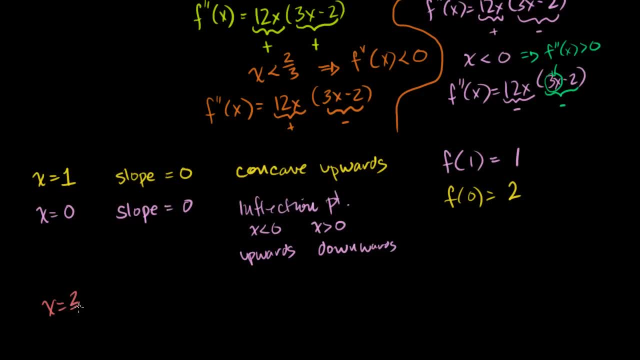 We had. the point x is equal to 2 thirds. We figured out that this was an inflection point. The slope isn't necessarily, or the slope definitely isn't 0 there, because it wasn't one of the critical points And we know that we are downwards. 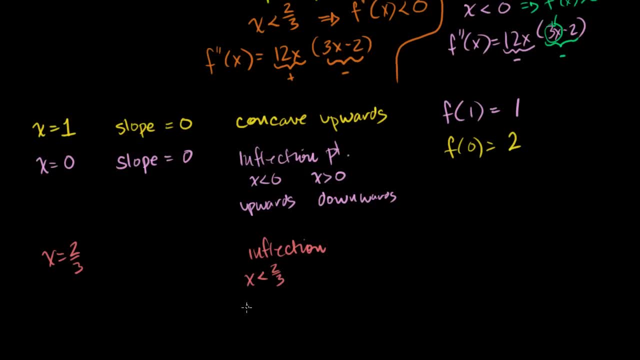 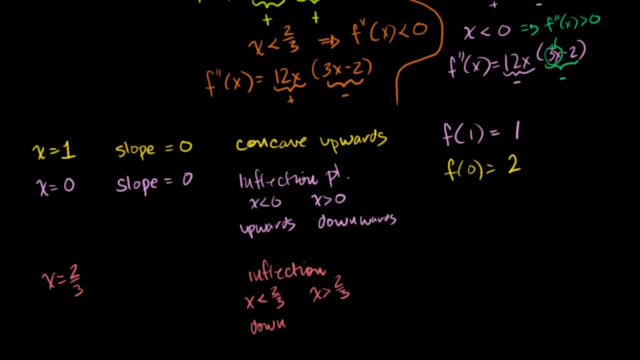 We know that when x is less than 2 thirds, or right less than 2 thirds, we are concave downwards, And when x is greater than 2 thirds- we saw it up here- When x was greater than 2 thirds, right up here. 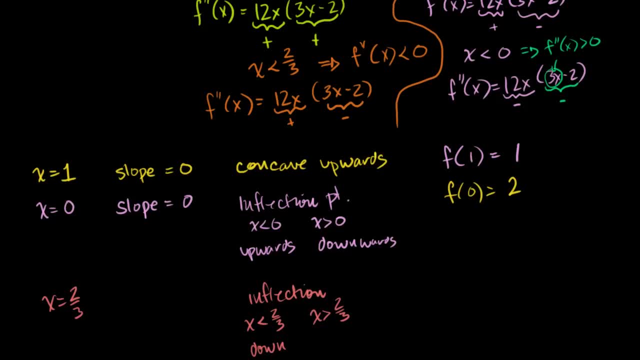 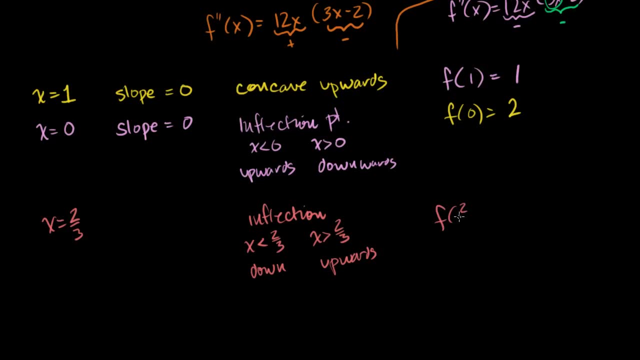 we were concave upwards. The second derivative was positive. We were upwards And we could actually figure out what's f of 2 thirds. That's actually a little bit complicated. We don't even have to figure that out. I don't think to graph. 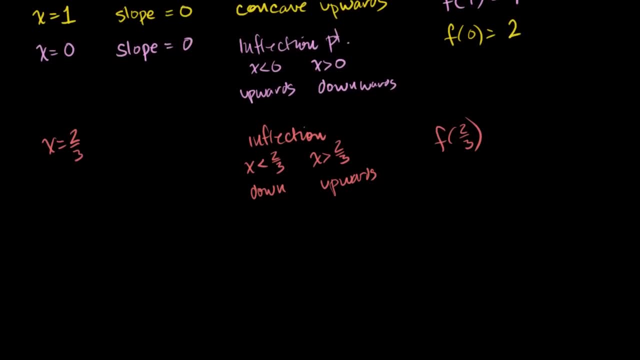 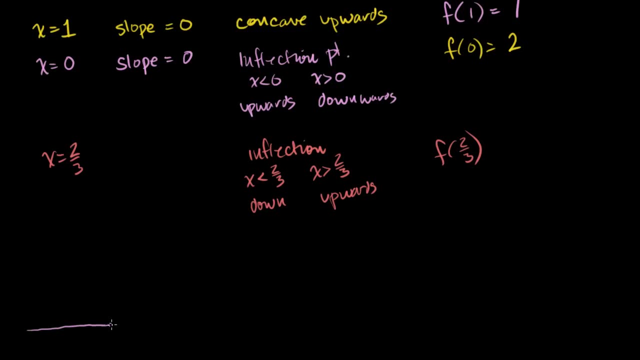 I think we could do a pretty good job of graphing it just with what we know right now. So that's our takeaways. Let me do a rough graph, Let's see. So let me do my axes just like that. 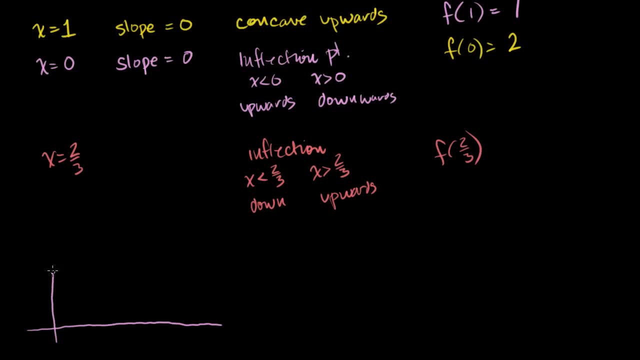 So let's see, we're going to want to graph the point 0, 2.. So let's say that the point 0, 2.. So this is x is equal to 0, and we go up 1, 2.. 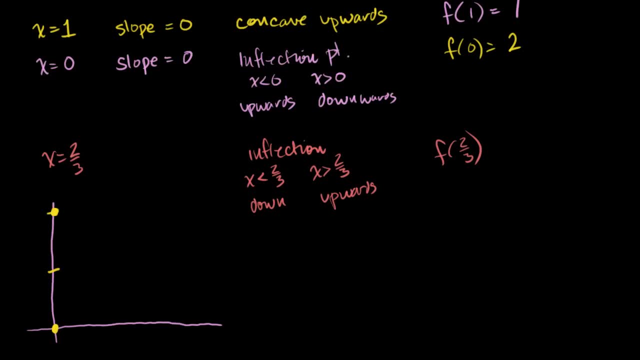 So this is the point 0, 2.. Maybe I'll do it in that color, the color I was using. So that's this color, So that's that point, right there. Then we have the point x, We have f of 1, which is the point 1, 1.. 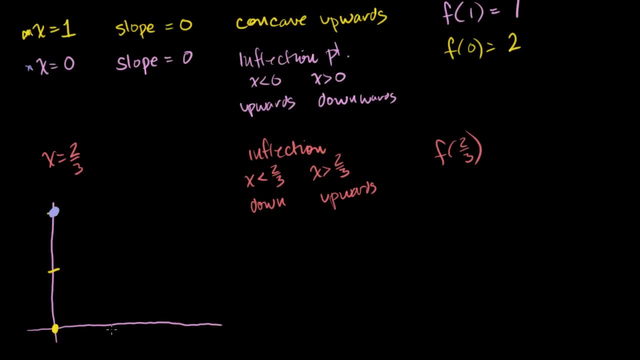 Right, So this is the point 1, 1.. Right, This point right here will go up: 1.. So that's the point 1, 1.. This was the point 0, 2.. And then we have: the x is equal to 2 thirds. 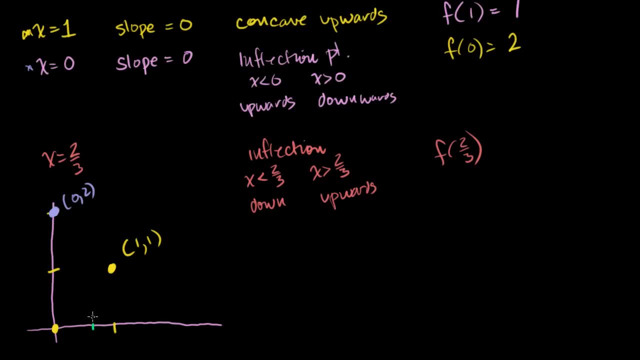 which is our inflection point. So when x is 2 thirds, we don't know exactly what number f of 2 thirds is. It might be here someplace. Let's say f of 2 thirds is right there. So that's the point: 2 thirds. 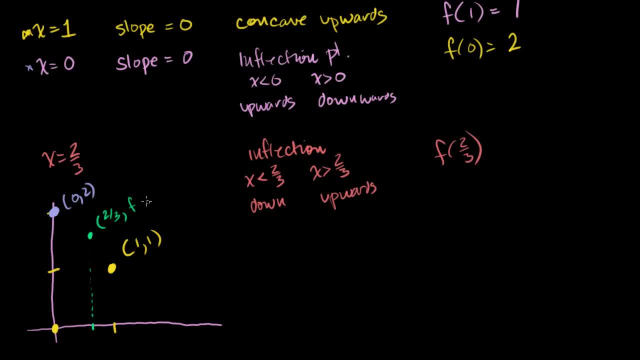 And then whatever f of 2 thirds is, it looks like it's going to be 1 point, something f of 2 thirds. You could calculate it if you like. You just have to substitute back in the function. But we're ready to graph this. 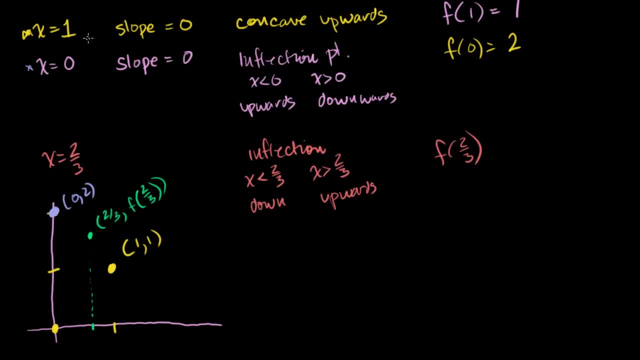 We're ready to graph this thing. So we know that at x is equal to 1, the slope is 0.. We know that the slope is 0.. It's flat here And we know it's concave upwards. So we're dealing. it looks like this: 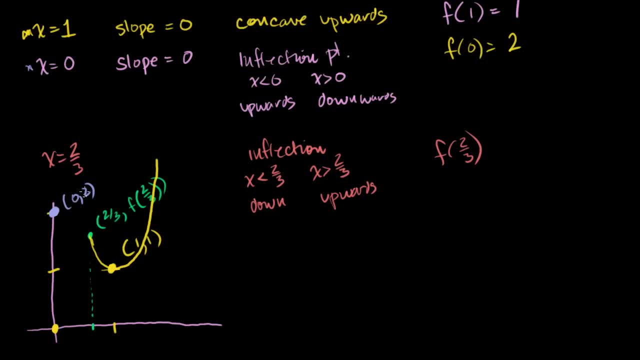 It looks like that over that interval We're concave upwards And we know we're concave upwards, from x is equal to 2 thirds, and on Right- Let me do it in that color We knew- x is equal to 2 thirds. 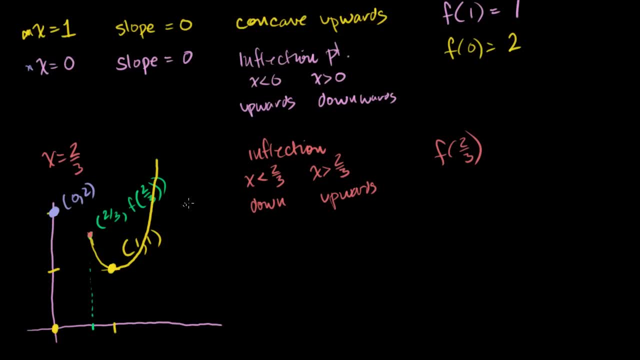 And on we're concave upwards, And so that's why I was able to draw this u shape. Now we know that when x is less than 2 thirds and greater than 0, we're concave downwards. So the graph will look something like this over this interval. 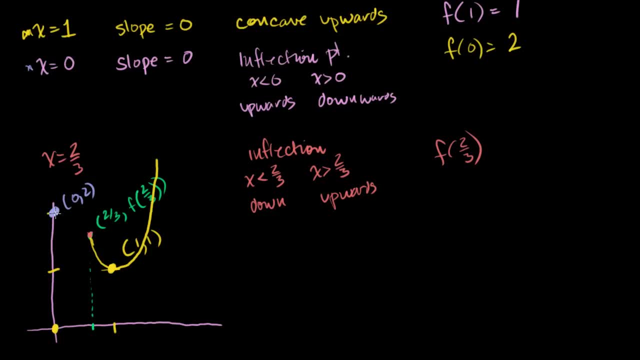 We'll be concave downwards. Let me draw it nicely Over this interval. the slope is decreasing And you could see it if you keep drawing tangent lines. It's flattish there. It gets negative, more negative, more negative, until the inflection point. 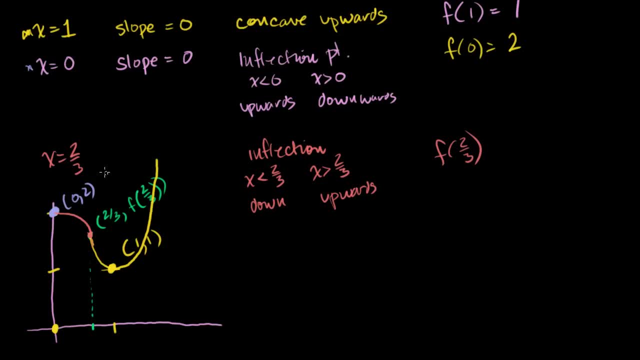 And then it starts increasing again, because we go back to concave upwards. And then finally, the last interval is below 0.. And we know below 0, when x is less than 0, we're concave upwards. So the graph looks like this: 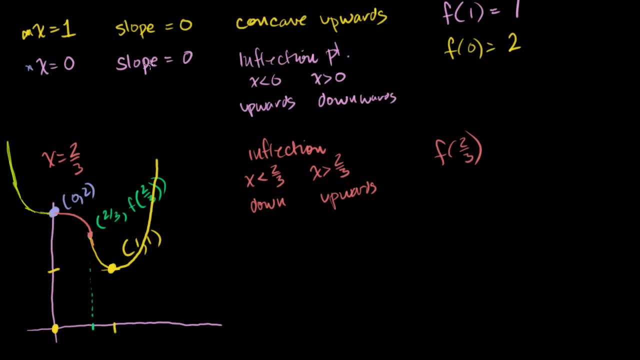 Well, the graph looks like that, And we also know that x is equal to 0 was a critical point. The slope was 0.. So this graph is actually flat right there too. So this is an inflection point where the slope was also 0.. 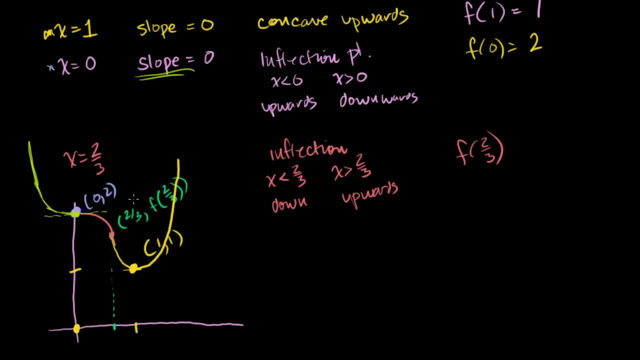 So this is our final graph. We're done. After all that work, we were able to use our calculus skills and our knowledge of inflection points and concavity and transitions in concavity To actually graph this fairly hairy looking graph. But this should be kind of what it looks like if you graph it. on your calculator.